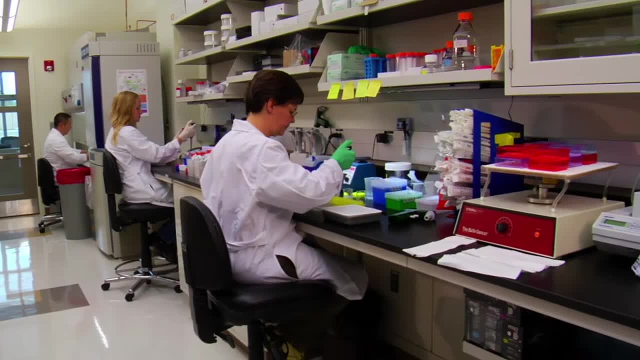 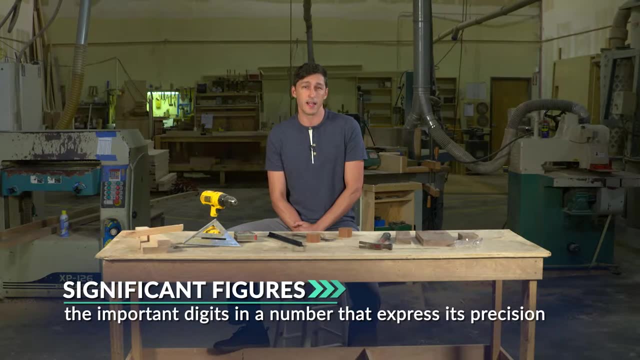 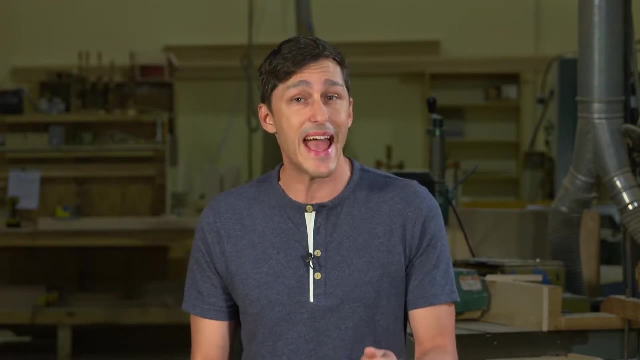 have guessed. yes, it matters, especially in Physics. Scientists have established a way of dealing with how precise a measurement is using significant figures. They are the important digits in a number, based on how exact you are when you report a number. Our instruments and tools are only exact to a point. They have limits In order to express. 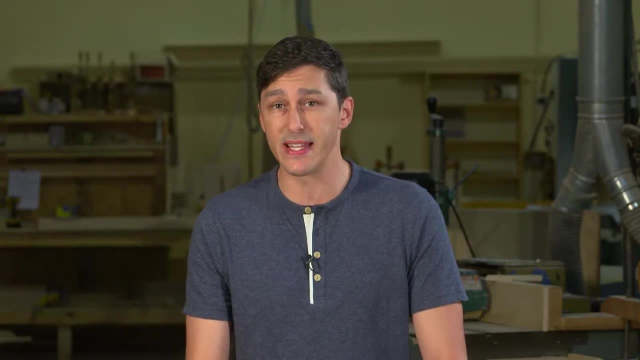 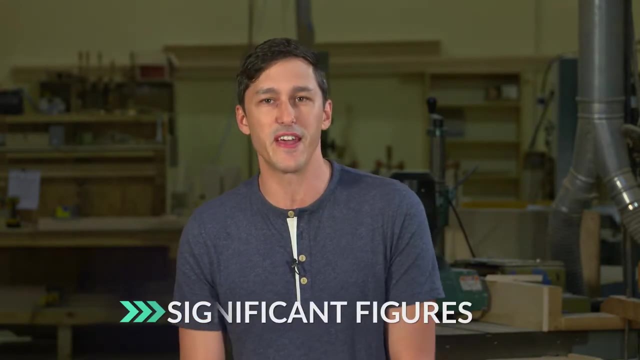 how exact we are being in our measurements. we need to decide which digits or figures are significant. That's what significant figures are. We often call them sig figs for short. Here are some of the rules we follow to do that. First of all, all non-zero digits. 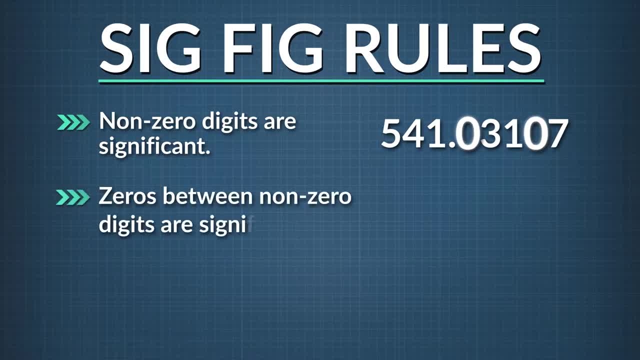 are always counted as significant figures. Any zeros between the non-zero digits are always significant. So that means these, the highlighted zeros, are sig figs, That's the two zeros in one, zero, zero four, The zero in between four and nine And final zero. 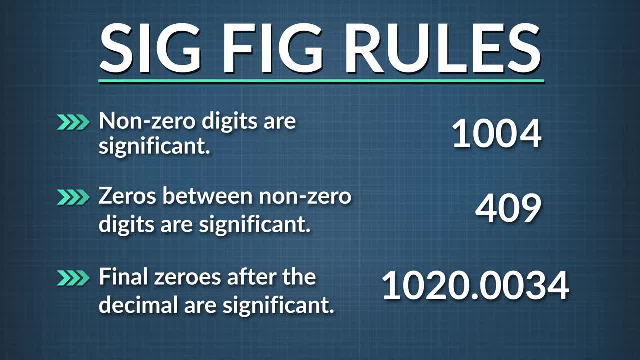 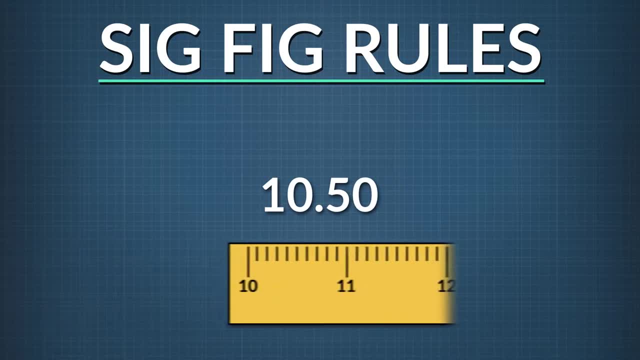 zeros in the decimal part of a number are also significant. These zeros are important because they show how exact our measurements are. For example, 10.50 meters says measured to the nearest 0.01 meter, And we verified that the object was not 10.51 meters or 10.49. 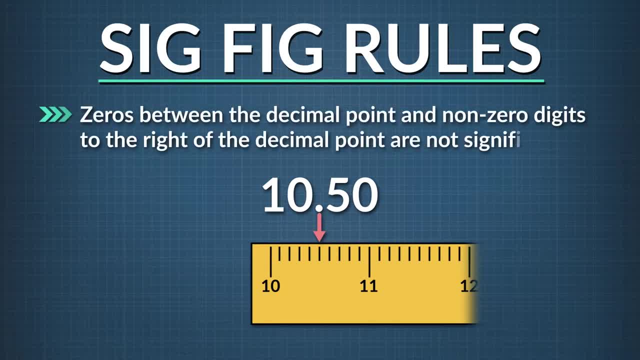 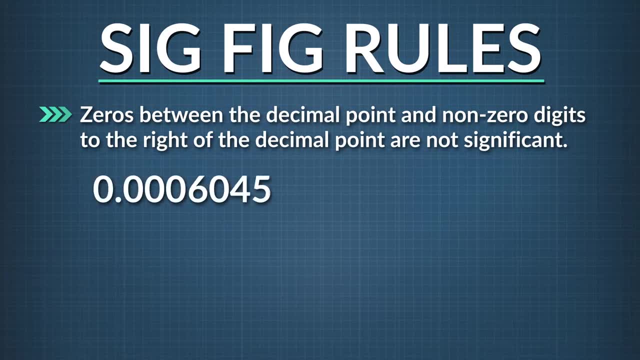 meters long, But zeros between the decimal point and non-zero digits to the right of the decimal point are not significant. For example, 0.00060450 has five significant figures. All those other zeros are not significant. 0.0100 has three sig figs and the other two zeros are not, And 0.00006010 has four. The 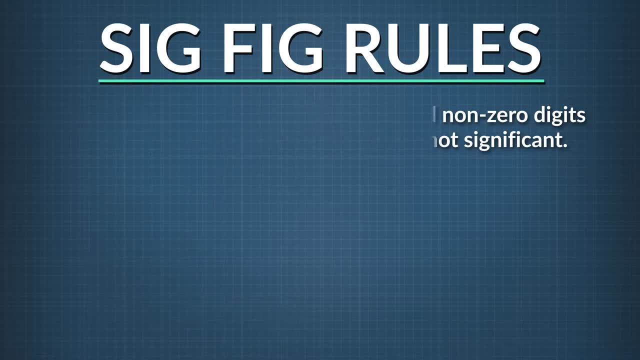 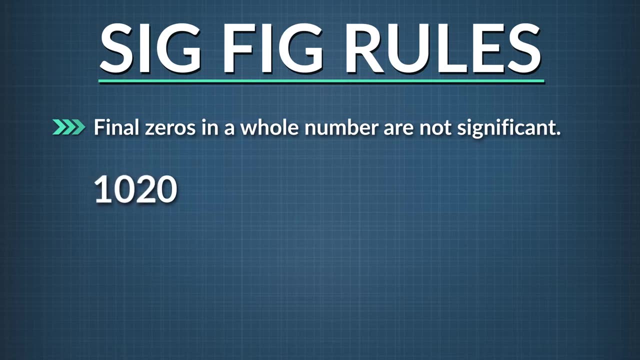 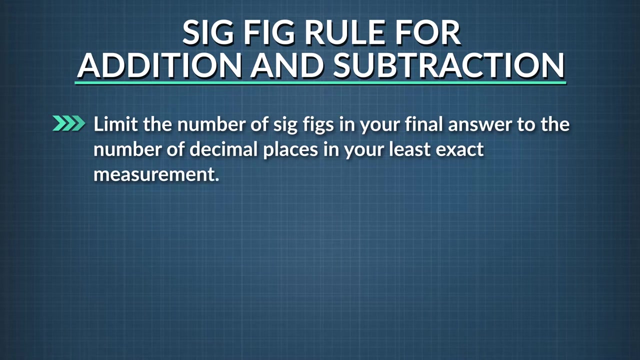 other five zeros again are not sig figs And final zeros in a whole number are also significant. 1.020 has three significant figures, 1.23000 has three significant figures And 1.203400 has five. Another rule to remember When you're doing addition and subtraction calculations: 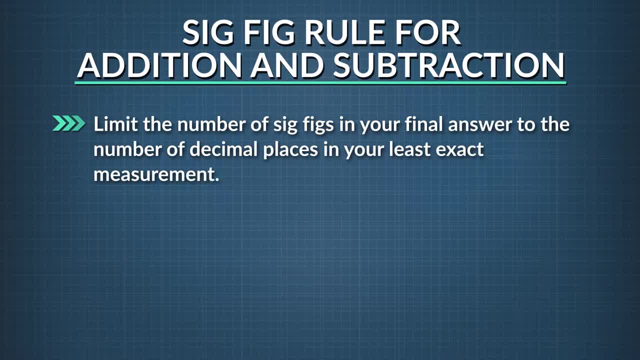 you limit the number of sig figs in your final answer to the number of decimal places in your least exact measurement. If your least exact measurement is a whole number, you're going to be able to measure the number of sig figs in your final answer. So your final 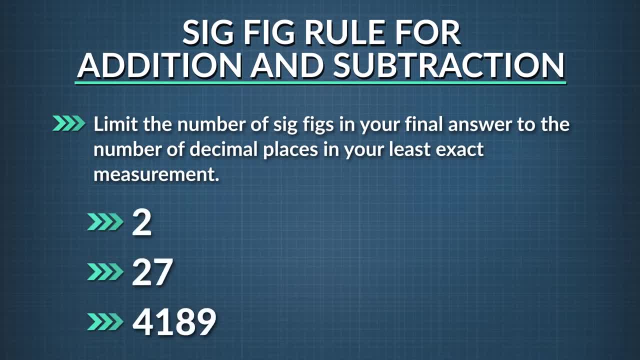 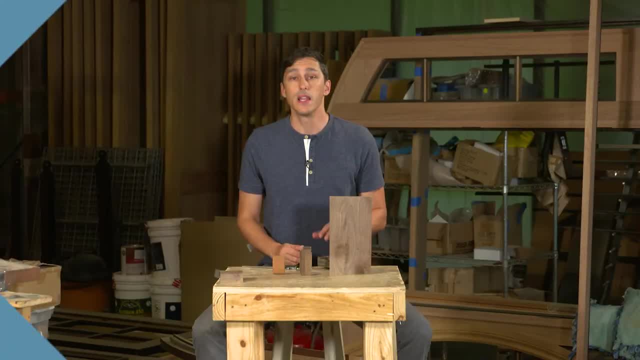 answer must be a whole number too. Or if your least exact measurement is to three decimal places, your final answer should also be to three decimal places. Let's do some measurements and we'll see where that rule comes into play. Let's say: 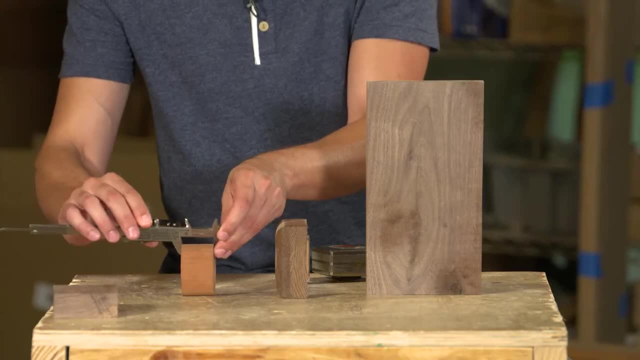 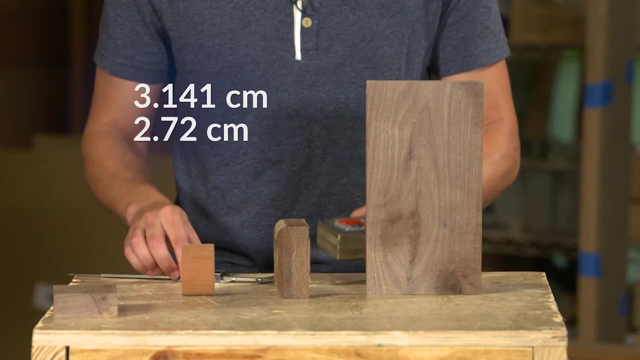 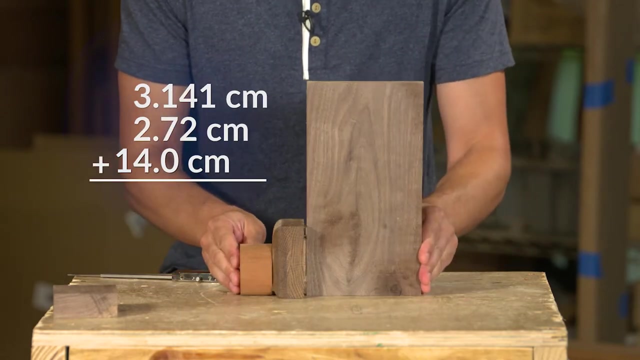 I measure these three pieces of wood. This one is 3.141 centimeters, This one is 2.72 centimeters And this one is 14 centimeters. So let's add those three up and we get 19.861.. And when adding or subtracting sig. 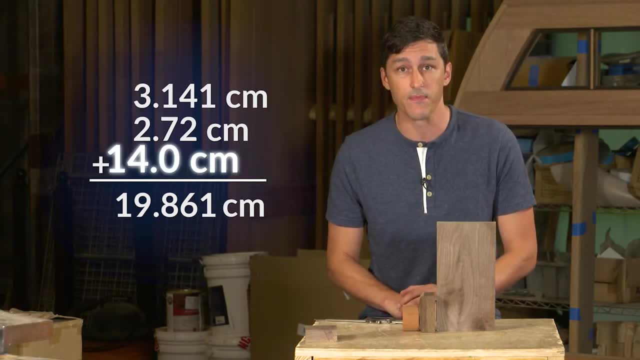 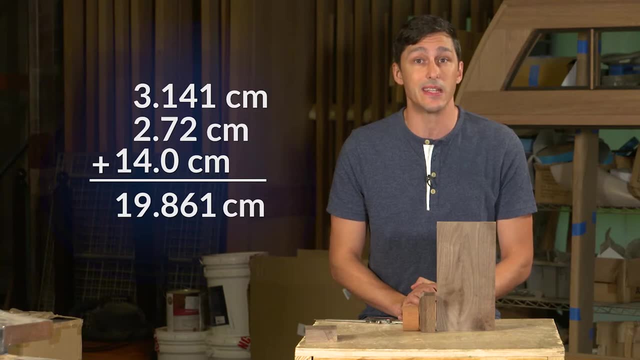 figs. I round to the least exact measurement, which is 14,, so I can have only one digit to the right of the decimal. However, 19.861 is closer to 19.9 than 19.8, so I will round. 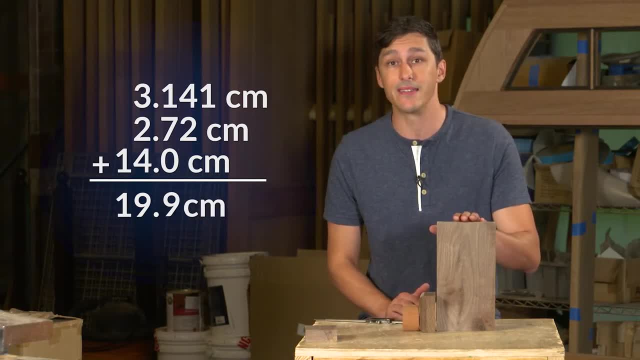 up. The correct answer is 19.9 centimeters. My total can only have one digit to the right of my decimal point Because of the 14.0.. So it would be 19.861, but we only want three sig figs. So our final. 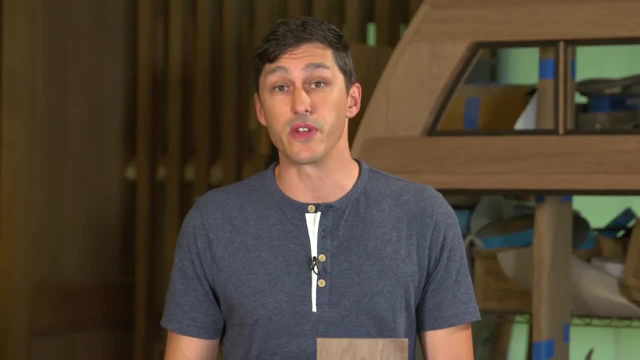 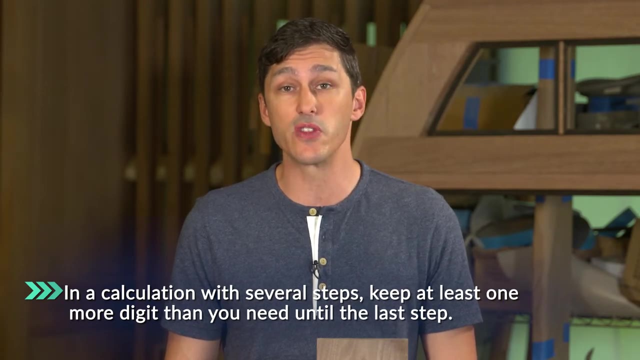 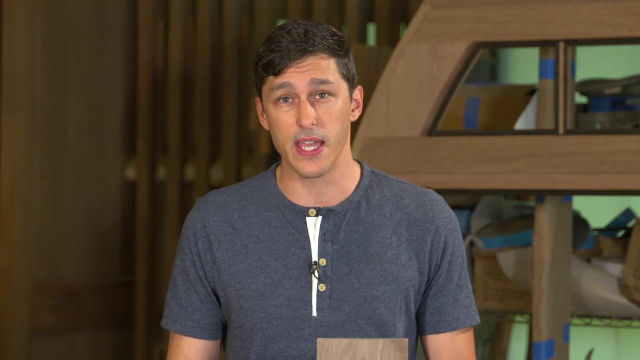 answer is 19.9.. One piece of advice: when you're dealing with sig figs, If you're doing a calculation with several steps, keep at least one more digit than you need until the last step. We do that because when we round numbers we lose some information If we keep the digits till the 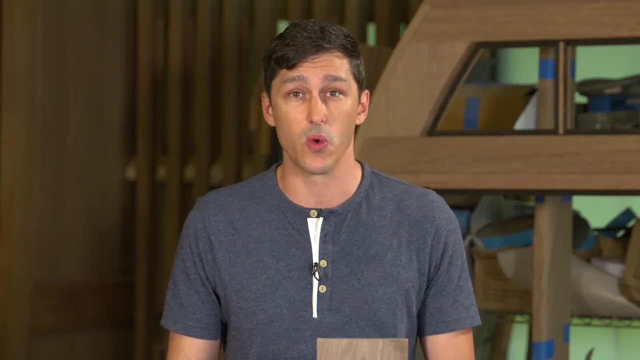 end we can make sure we're not losing more information than we want to before we get to the final answer. When you do multiplication and division, it's a slightly different rule from addition and subtraction, where you have to line up the decimal points. So for multiplication and 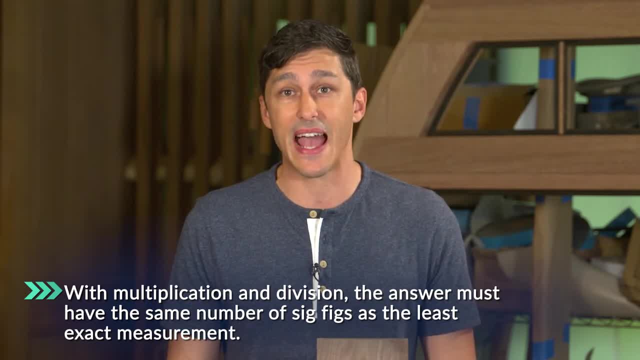 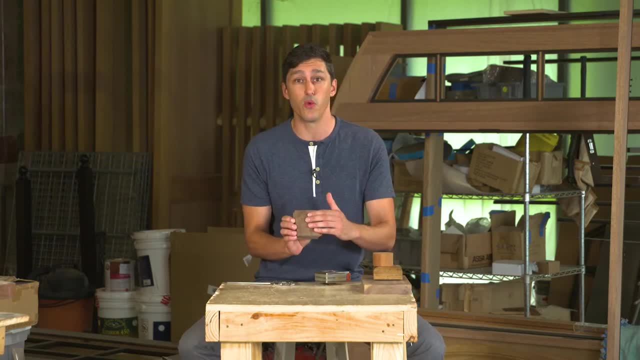 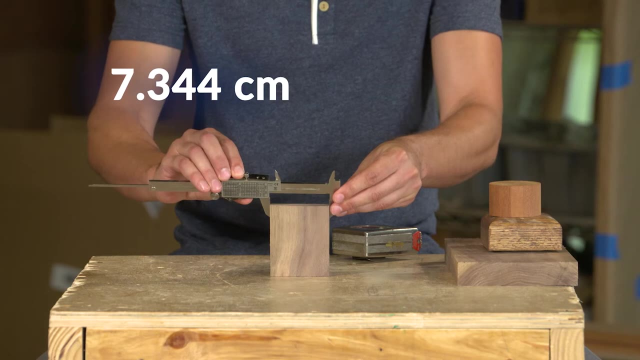 division. the answer must have the same number of sig figs as the least exact measurement. Let's see how that works. Suppose we are measuring the top of this piece of wood and we want to determine the area of the surface. The width has four significant digits: 7.344 centimeters.